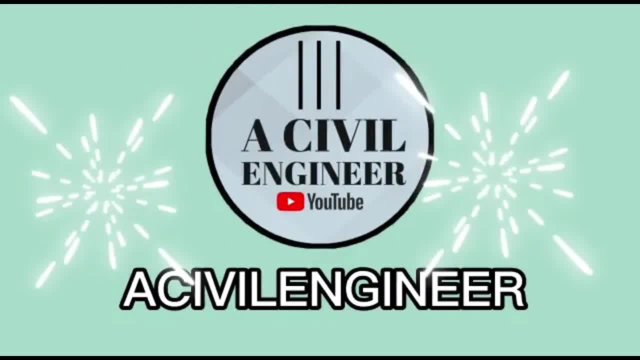 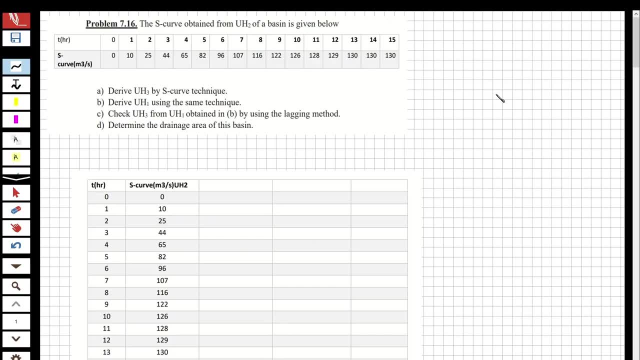 Hi guys, welcome to my channel. In this video we are going to solve the questions about engineering hydrology, and the question will be from the chapter of hydrograph analysis. So now let's solve the question. But before we solve the question, if you like these videos, 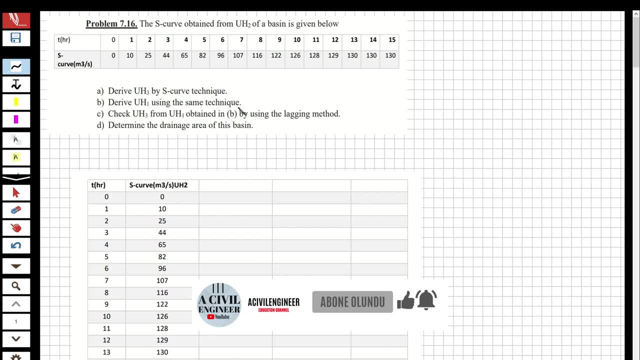 if you want to see more of the videos, please subscribe and share with your friends. So now let's pass the question. The first: the s-curve obtained from the unit hydrograph for two hours of a basin is given below. Now you can see here for s-curve and we are going. 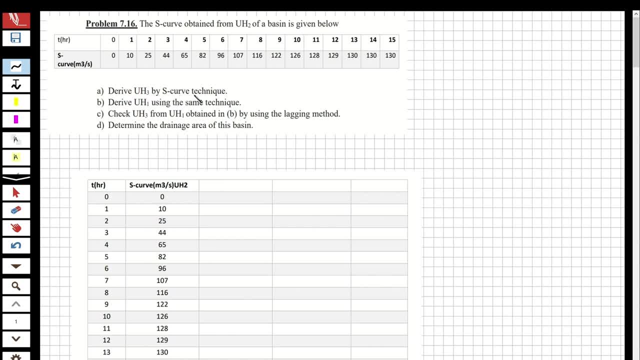 to derive the unit hydrograph for three hours by s-curve technique. So let's do it First. I'm going to show you here for the A. Ok, this is going to be for A. So now we have an s-curve here. We have an s-curve here for two hours: unit hydrograph. So now I'm going to lag it. 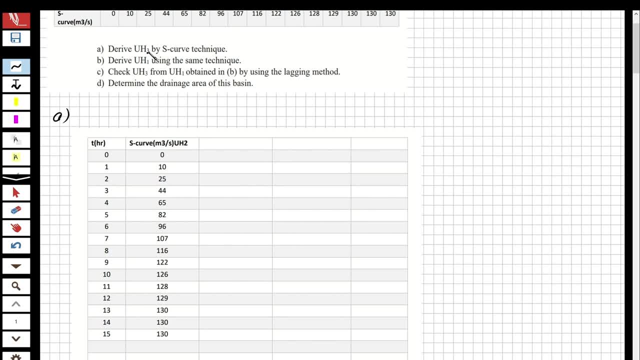 for three hours. Look at here, because it asks as three hours, So I'm going to lag it for three hours. This is one second. Three hours lagged, Ok, And it's going to be three hours lagged and it's going to start with here: Zero, Ok, Ten And twenty-five and forty-four and sixty-five. 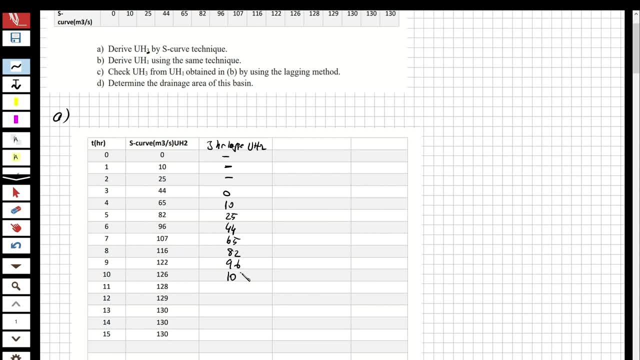 And ninety-six, and it's going to be one hundred seven, and it's going to be one hundred sixteen and one hundred twenty-two and one hundred twenty-six and one hundred twenty-eight, One hundred twenty-nine and one hundred thirty. Ok, So now we got it. So let's take the differences. 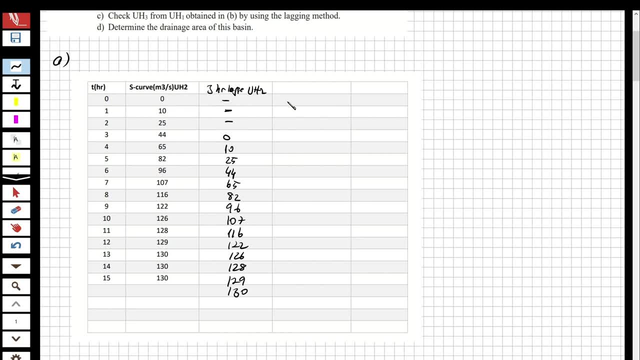 of this, both column. Ok, Take the differences of them. We are going to take the differences. So, from the differences, it's going to be zero, It's going to be ten and this is going to be twenty-five. Right, This is going to be. 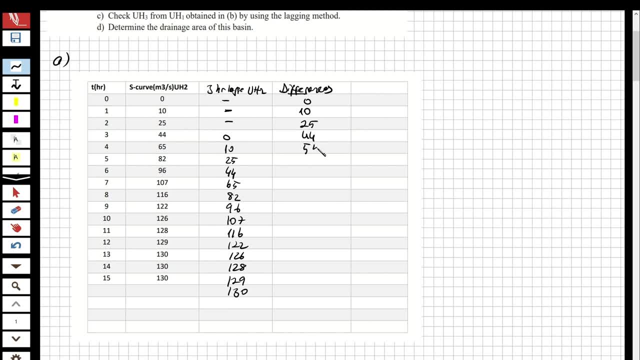 forty-four, and this is going to be fifty-five, and this is going to be fifty-seven. This is going to be forty-two, Sorry, fifty-two, And this is forty-two, and this is thirty-four, And this is twenty-six, Nineteen And twelve. It's going to be seven And this is going. 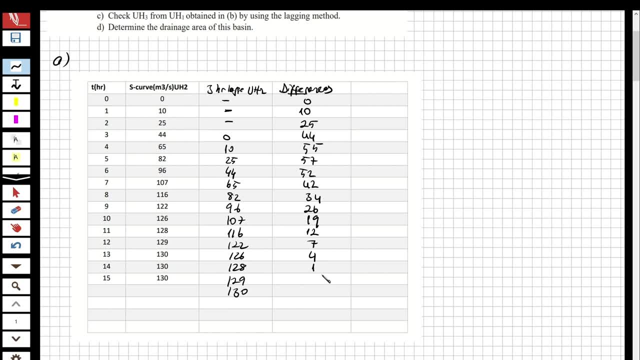 to be four And this is going to be two, And this is going to be one And this is going to be zero. Ok, So now we got the differences of this both column, Ok. For example, this is A and this is B. We are like: this is A minus B. Ok, 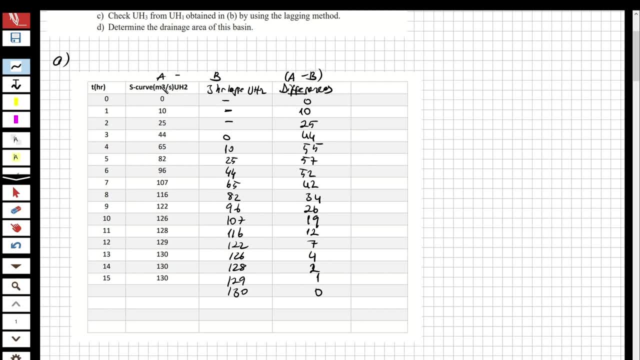 Now we are going to multiply the differences of this. both columns with the ratio: Ok, This ratio, this ratio is going to be this one. For example, now it is given as two hours unit hydrograph, Right. So we are going to write the up of the line as two: Ok. And for the 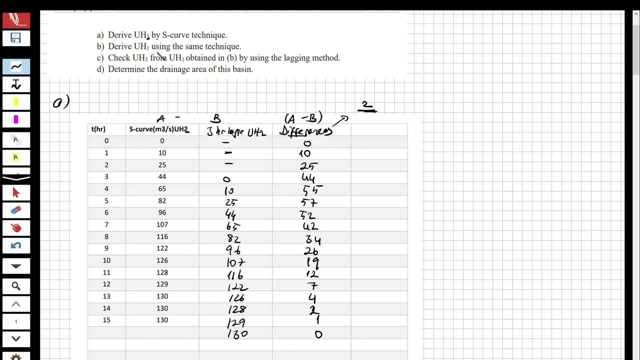 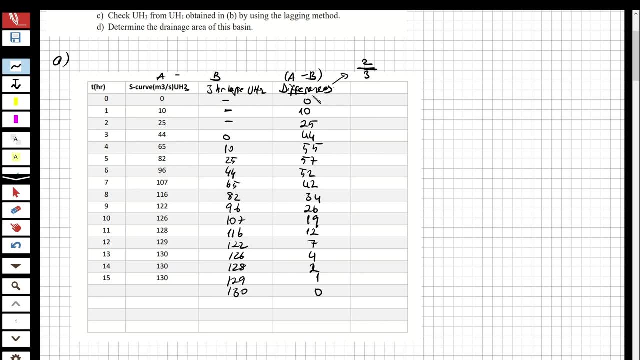 bottom. we are going to write as which one it asks In the question. it ask three hours unit hydrograph, Right, So it's going to be two over three. okay, i'm going to multiply the differences with the two over three and i'm going to obtain. 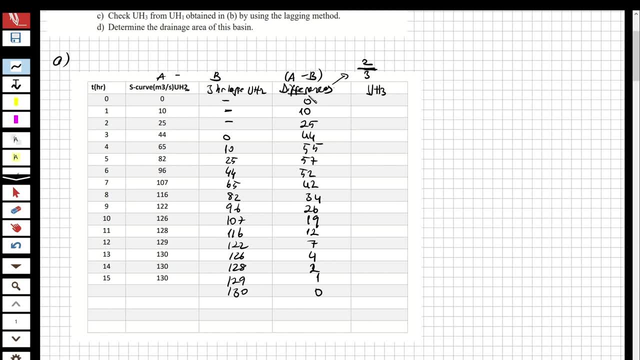 as unit hydrograph for three. okay, so let's do it. it's going to be zero and 10 multiplied 2, 20 over 3 and it's going to be 6.67. right, and it's going to be 16.67. it was 25 multiplied 2 over 3. it's going to 16.67. 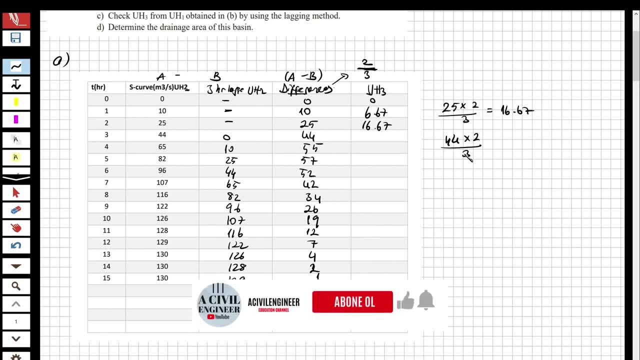 and 44, multiply 2 over 3 and it's going to be 29.33. okay, so it's going to be multiplied with this ratio and this is going to be 29- sorry, yeah, 33 and 36.67 and 38, 34.67, 28,, 22.67, 17.33, 12.67, 8, 4.67, 2.67,. 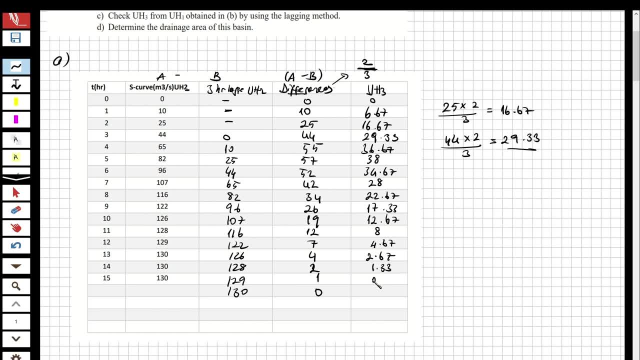 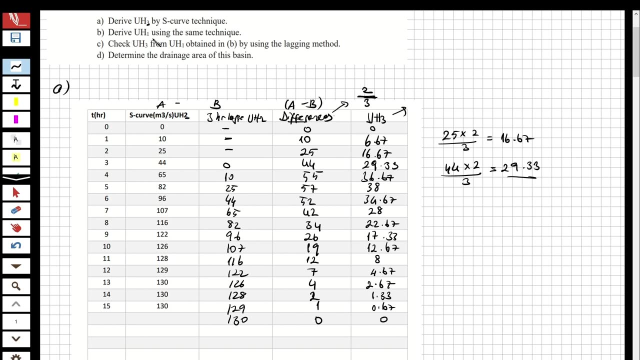 1.33, and 0.67, and 0.. Now we got the unit hydrograph for three hours. The part of A is solved, So let's solve the part B And we are going to derive the unit hydrograph for one hour, okay. 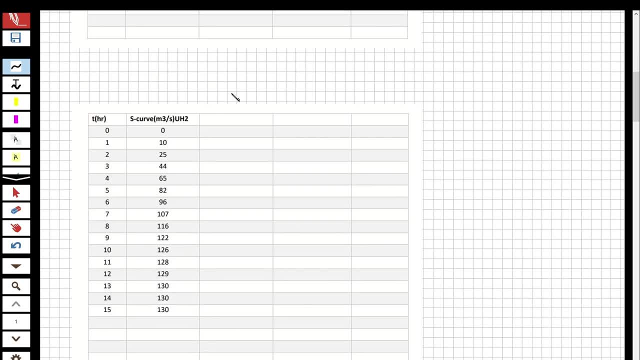 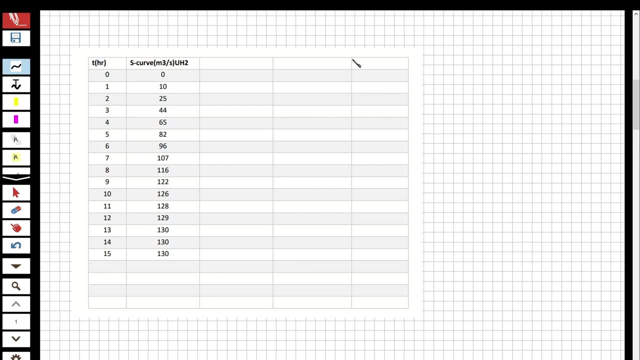 Using the S-curve technique. So now let's do it for the unit hydrograph one hour. So how it's going to be? For the previous part, we lagged three hours for the unit hydrograph three, okay. So now we are going to lag one hour for unit hydrograph one, okay. 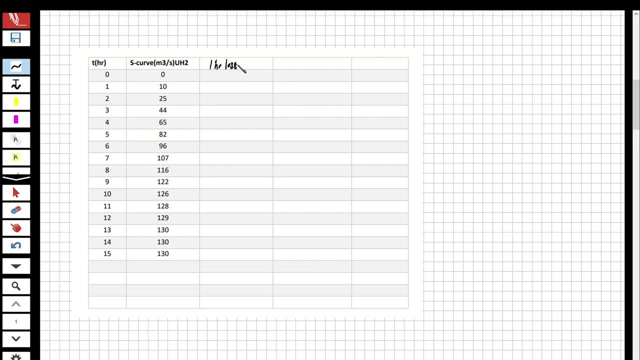 One hour. one hour lagged for unit hydrograph one right, So we are going to lag it for one hour. So it's going to be there will be no any flow here, so it's going to start with this row, okay. 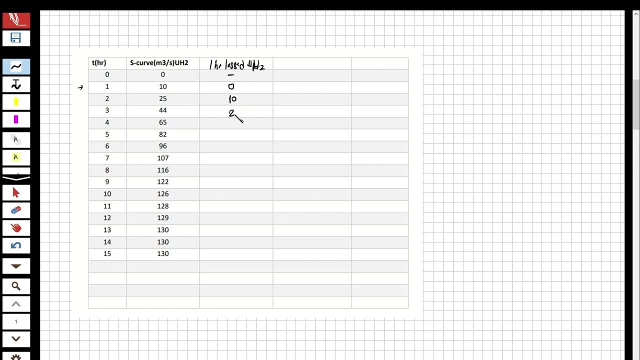 And with zero, and it's going to be 10, and 25,, 44,, 65,, 82.. And this is going to be 96, and 107,, 116,, 122,, 126,, 128,. 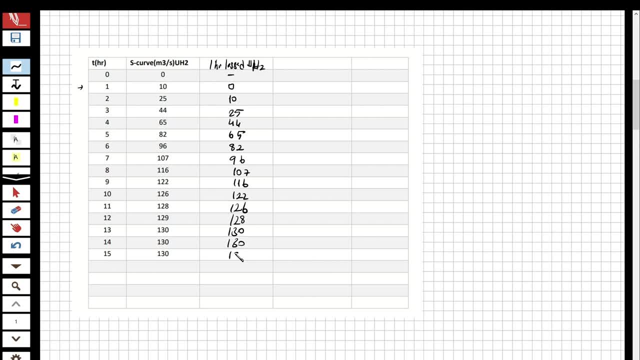 130,, 130, 130.. Now, it's okay, We got the one hour lag unit hydrograph for two hours. So now we are going to take the differences of both because you know, for the S-curve we have to take the differences okay. 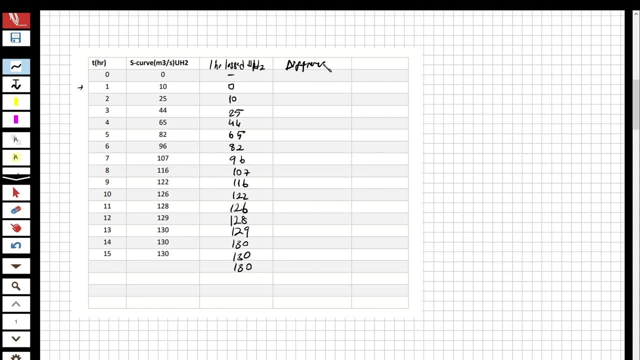 So it's going to be differences. Let's take the differences: This is zero, this is 10,, this is 15,, this is 19, and this is 21,. this is 17,, this is 14, and this is 11,. okay. 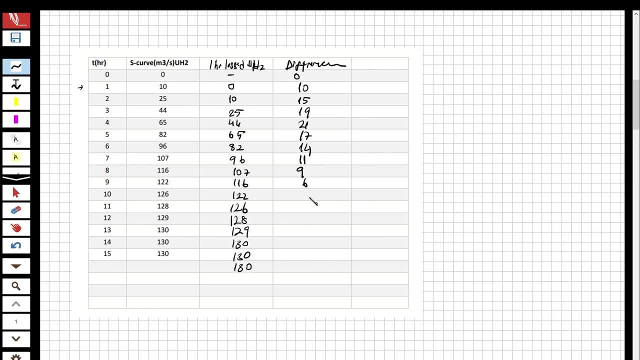 And this is nine, six four, two, and this is going to be one, and this is going to be one and this is zero. okay, So now I guess you remember. for the previous, I told you that we have to multiply. 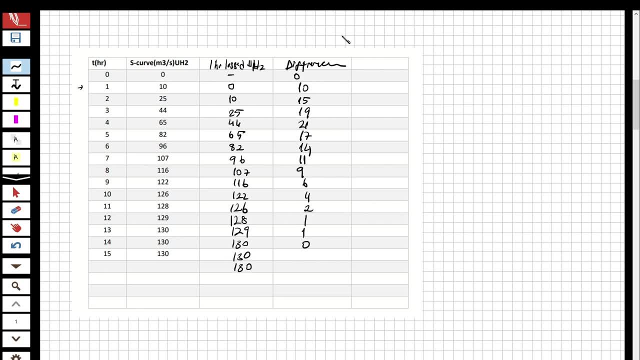 multiplied the differences by a ratio. okay, So what was the ratio? What was the ratio? The given unit hydrograph is for two hours. okay, This one for two hours, And the question is asked for the one hour unit hydrograph. 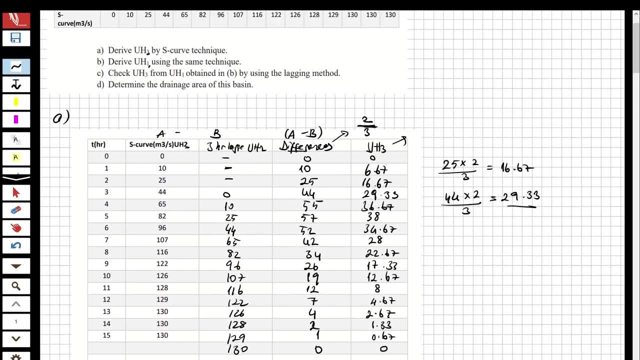 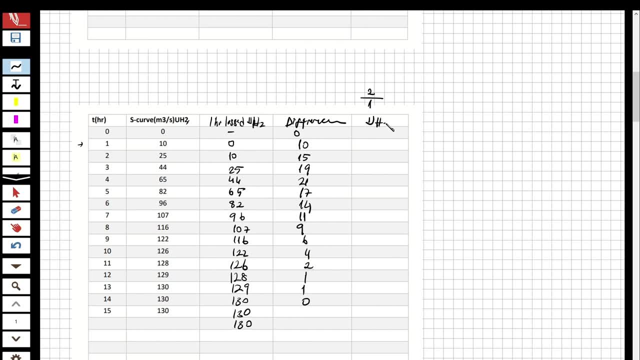 If you remember, look at here for the question- for one hour. So it's going to be two over one, right, Two over one. So this is going to be unit hydrograph, So the unit hydrograph for one hour. So now I'm going to multiply. 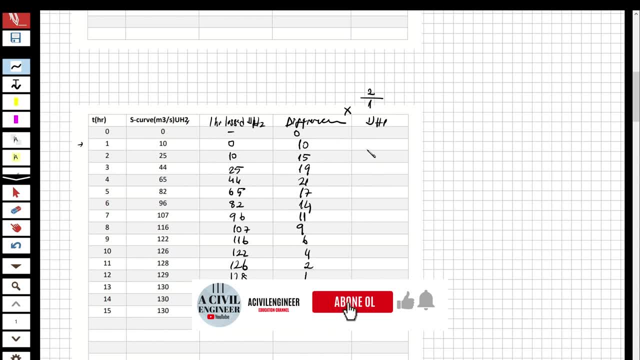 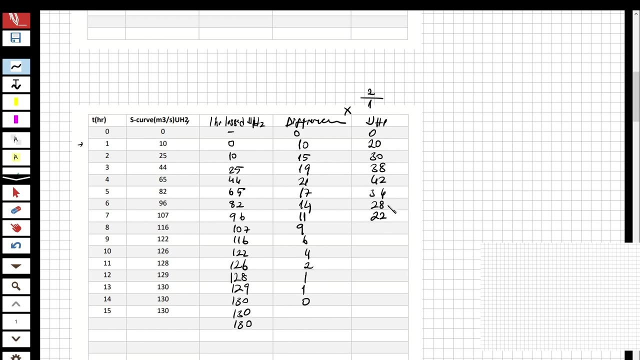 I'm going to multiply the differences with this ratio. So let's multiply. it's going to be zero, 20,, 30,, 38,, 42,, 34, and this is going to be 28,, and this is going to be 22,, and it's going to be 18,. 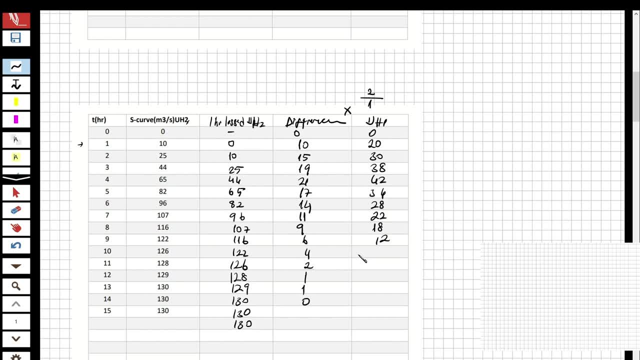 this is going to be 12, and this is going to be eight. this is going to be, uh, four, sorry four, and it's going to be two, and it's going to be two and it's going to be zero. so now you can see that i got the entire door for one hour. this was the part b. 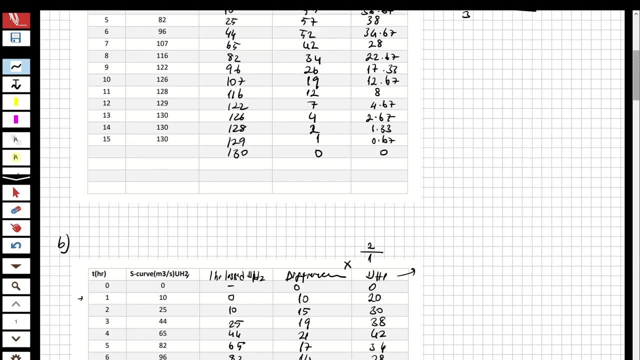 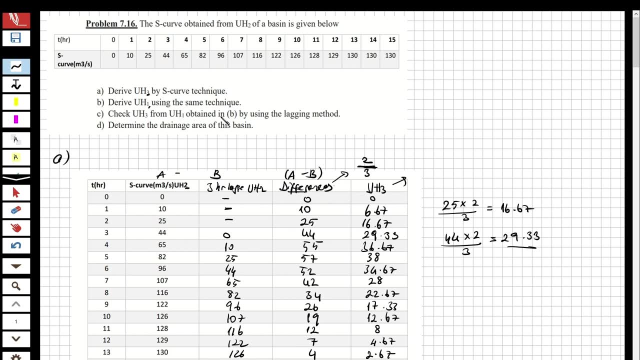 so we also saw the for part b. so let's check for the uh part c. what it asked: check unitary over three, four, sorry, from user for one obtained in b. okay, by using the lagging method. so now we are going to use the unit hydrograph one and we are going to obtain unit unit hydrograph three and we 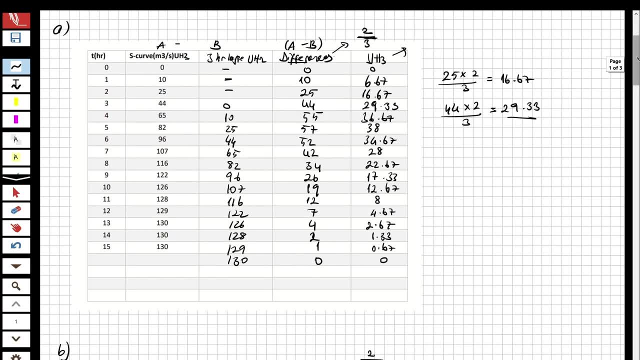 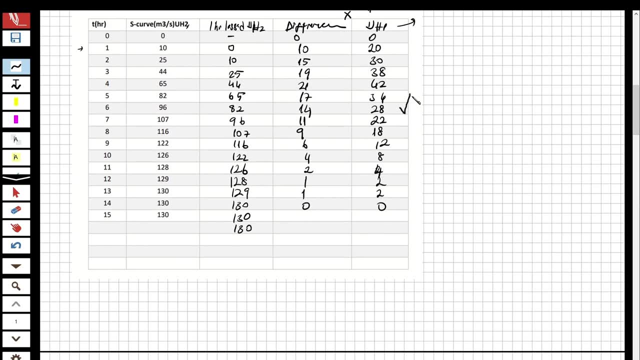 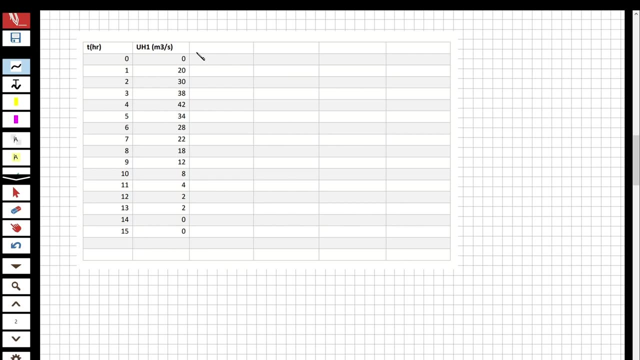 are going to check that they are the same. this one, so let's do it. look at here. i have this unit hydrograph of one hour here, okay, so now i'm going to take this one and write it down here. so now let's do it for the c, the part c. this is going to be part c. 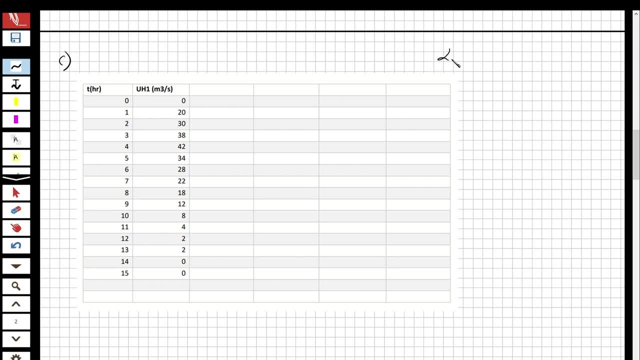 this is unit one for one hour. by lagging methods. by lagging method, we are going to determine unit hydrograph for three. okay, so how it's going to be if i lag one by one? sorry, look at here. one hour, unit hydrograph one, and again i'm going to make another, make another lagging for two hour. right, two hour. 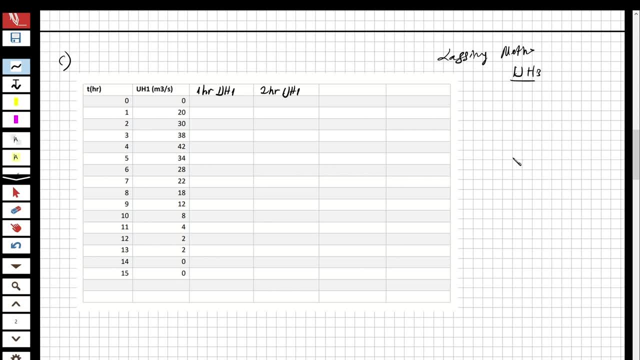 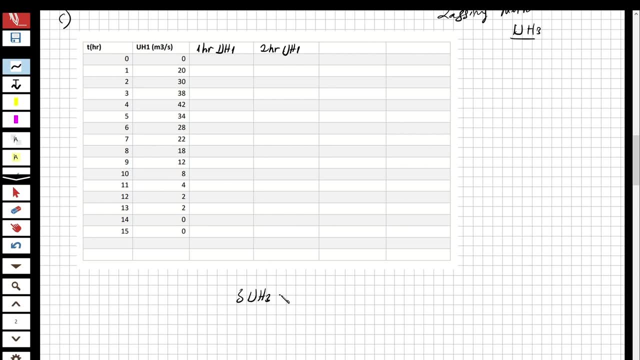 unit hydrograph one, because i i'm going to give you formula before, so it's going to be better for you. three hour unit hydrograph three is equal to unit hydrograph one plus one hour unit hydrograph- sorry, a one hour lagged. one hour lagged, unit hydrograph one and plus two hour lagged. 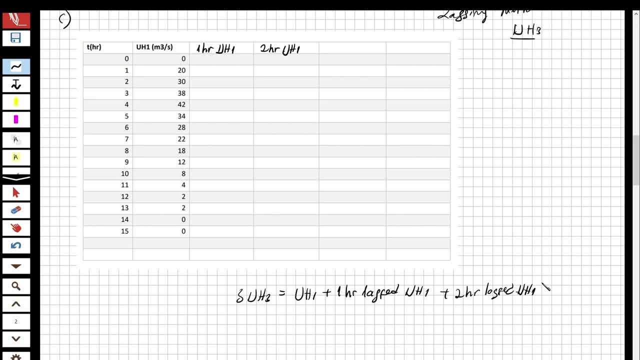 unit hydrograph one and this three. when i take the summation of this three, i'm going to obtain the three unit hydrograph three, and i have to divide it three. okay, to obtain the unit hydrograph three. so let's do it. i'm going to lag it one hour lagged. 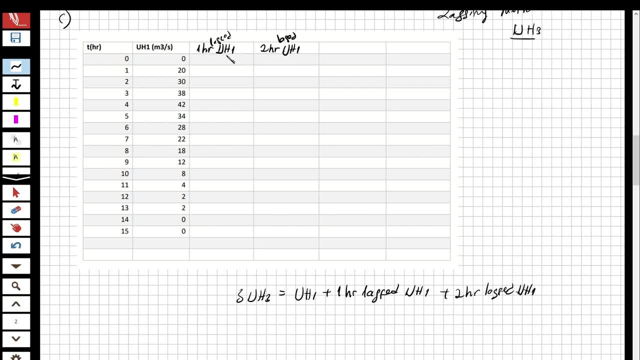 and two hour lagged. so first i'm going to do, if i'm going to do, for this one, one hour lag. this is going to be: there is no flow and it's going to be zero and it's going to be 20 and 30 and 38. 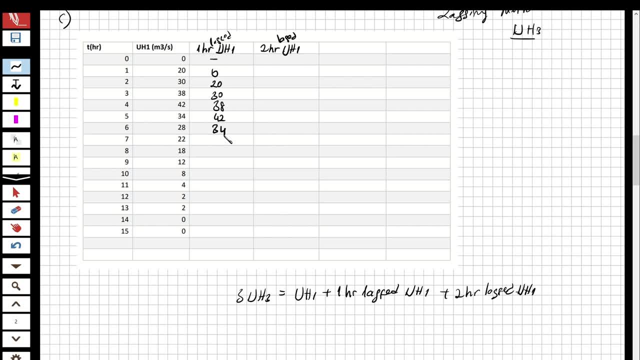 and it's going to be 42, and it's going to be 34, 28, 22, 18 and it's going to be 12, 8, 4, 2 and 2. okay, now we obtain this all, so let's do it for the two hour lagged unit, hydrograph one. this is going to be: 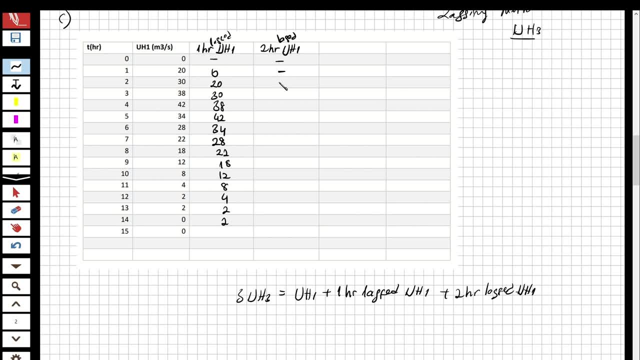 there will be no a flow. there will be no flow. and here we are going to start. it's going to be 0, 20 and this is going to be 30. it's going to do 38, 42, okay, 34, 28, 22, 18. 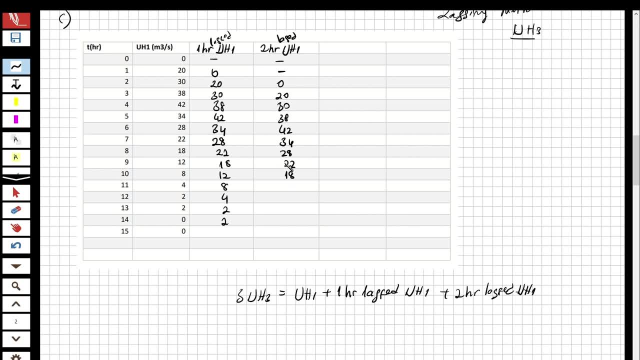 uh, i wish i didn't make any mistake. no, no, it's okay, it's correct. so this is going to be 12, it's going to be eight, it's going to be four, it's going to be two and it's going to be two. now we got it. these are zero. 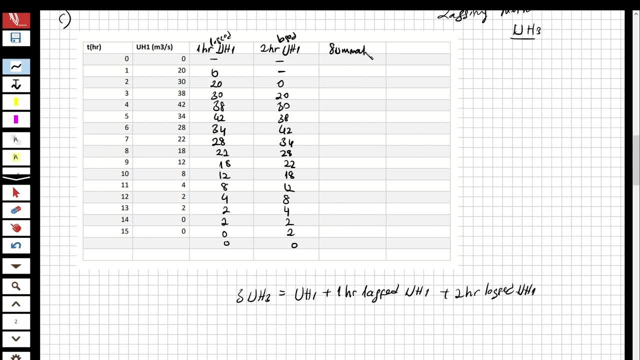 and now i have to take the summation of them. okay, summation. so when i take the summation of them, it's going to be something like that: this is going to be 0, this is going to be 20 and this is going to be i'm going to. 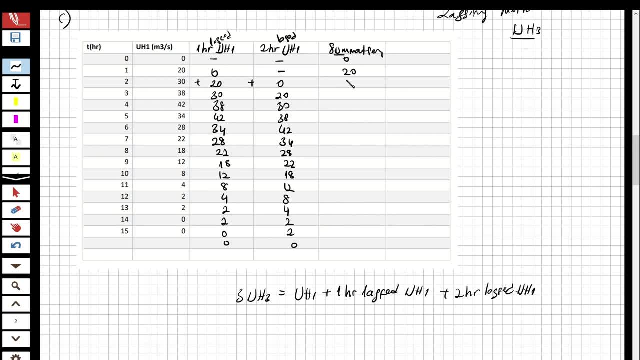 take the summation of them right: 30, 20, 50 and 30, 30 and 20, it's going to be 88, this is going to be 110, 114 and 104 and 84 and this is going to be 68, 52 and this is going 38. 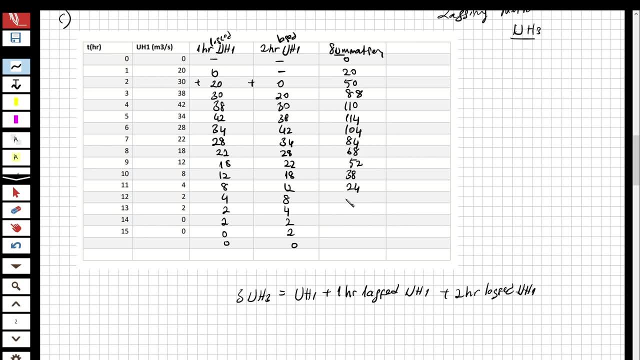 30, 24, and this is going to be 14 and this going to be 8, it's going to be 4 and it's going to be 2, it's going to be zero. so now we got the summation of them. so now i told you that. i told you that. 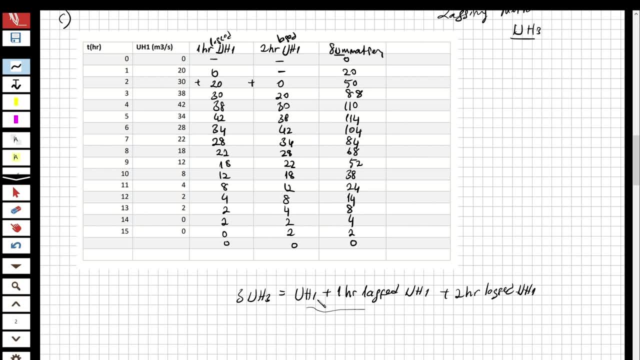 look at the formulation. i got the summation of one hour unit hydrograph, okay, and then one hour lagged for one hour unit hydrograph. this one, okay, look at it. this, this and now the third one is this one: two hour lagged, one hour unit hydrograph. so i take the summation of them and this is equal to: 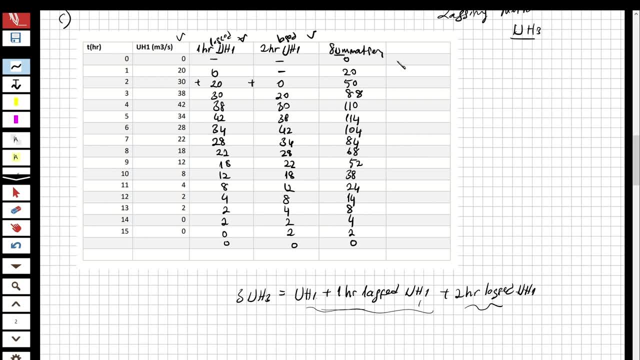 three hours. unit hydrograph for three. so now let's so. uh yes, three unit hydrograph for three hours. yeah, three hour. three unit hydrograph for three hours. so let's divide this summation, summation over three, and we are going to obtain unit hydrograph for three hours. so now let's do it. 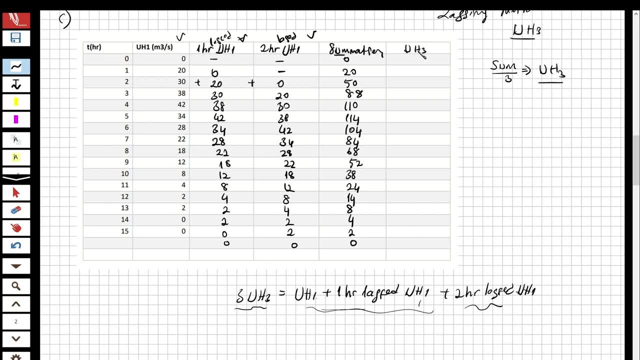 and this is going to be 20, and this is zero, and this is going to be 20 over 3, 6.67, and 50 over 3, and this is going to be 16.67. okay, so now let's write it. you understand how we are going to do it, but then we need to. 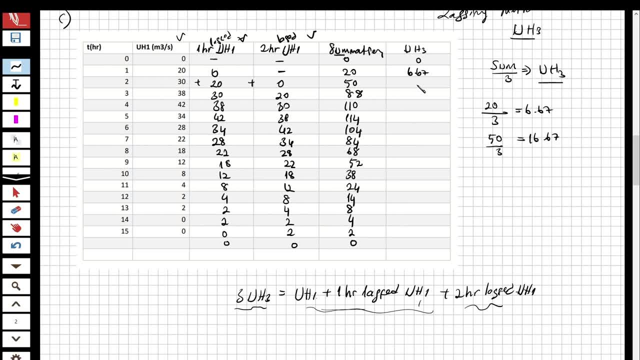 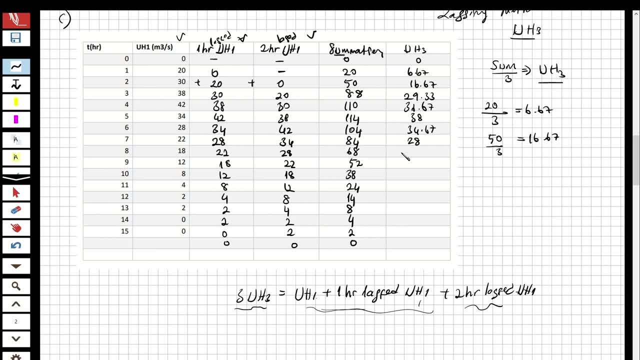 thirty four point thirty four point sixty seven, sixty seven, sixty seven, twenty eight, twenty eight, twenty eight, twenty two point sixty seven and twenty two point sixty seven and twenty two point sixty seven and seventeen point seventeen point seventeen point thirty three, thirty three, thirty three and twelve point sixty seven. sorry, yes. 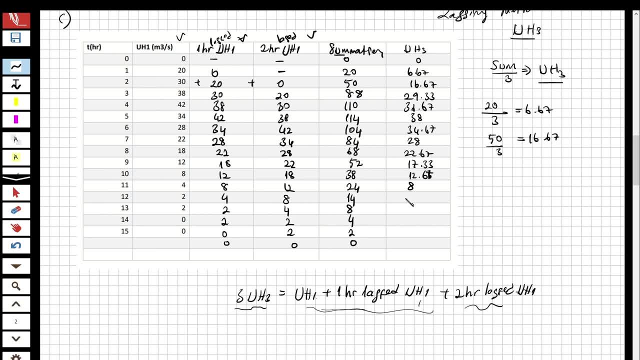 and twelve point sixty seven, sorry yes, and twelve point sixty seven, sorry yes. sixty seven, sixty seven, sixty seven and eight and eight and eight. four point sixty seven, four point sixty seven, four point sixty seven. two point 1.33 and 0.67 and 0. now you can see that we got the unit. 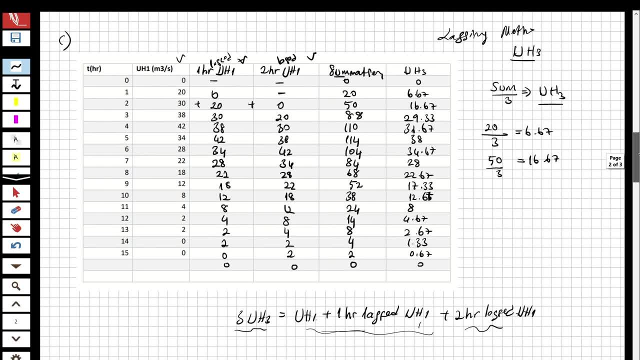 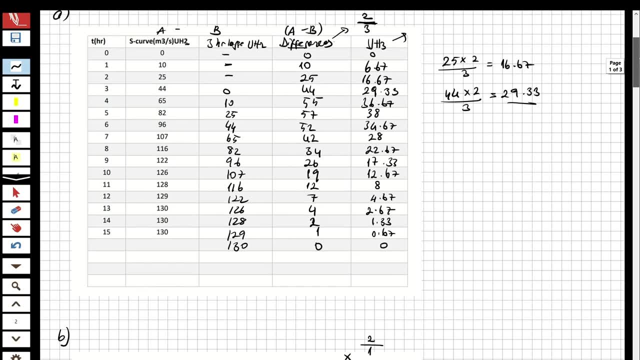 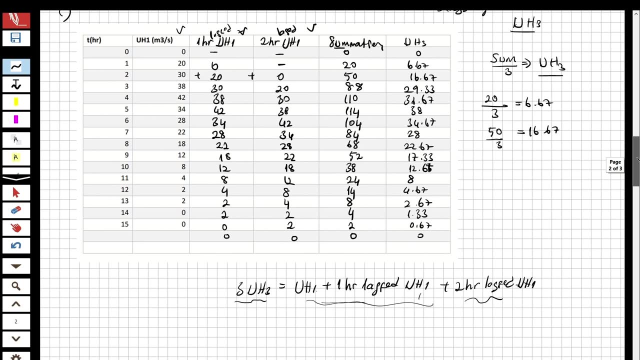 hydrograph for 3 hours. so let's, we are going to make a check with the first one. look at here: 6.67, 16.67. it is the same with the new unit hydrograph for three hours that you obtained, so the result is the same. okay, so the part C is. 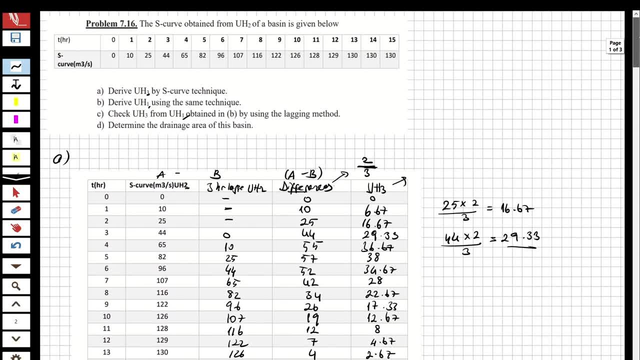 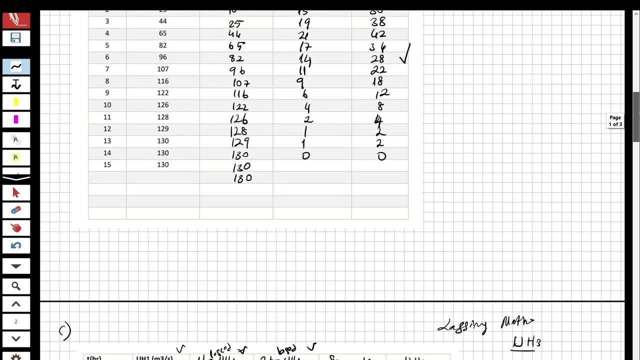 also solved. so let's solve the part 4. it says that determine the drainage area of the basin. so how it's going to be determined, let's think about it. look at here now we have unit hydrograph for one hour. okay, if you want to, if you want to. 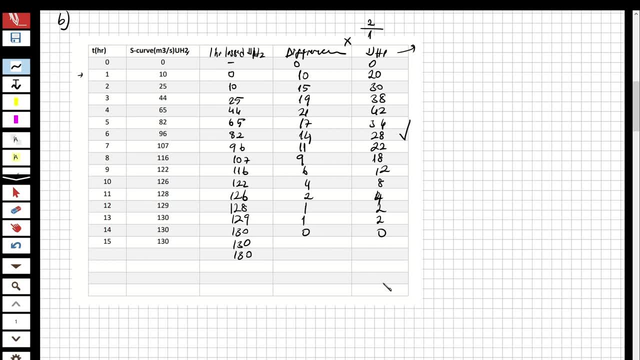 calculate the drainage area, you have to take the summation of unit hydrograph for one hour. okay, so now I take the summation of that. summation of this. all you are going to obtain as 260, 60 meter cubic per second as the discharge. okay, 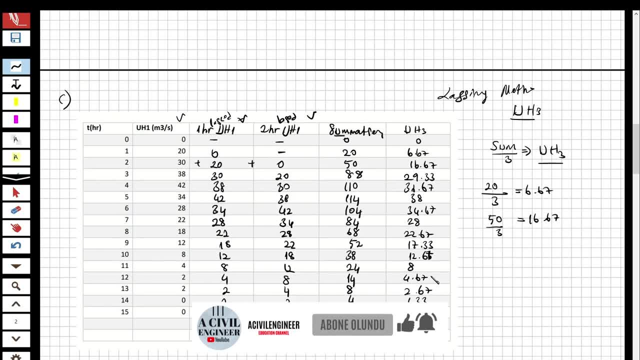 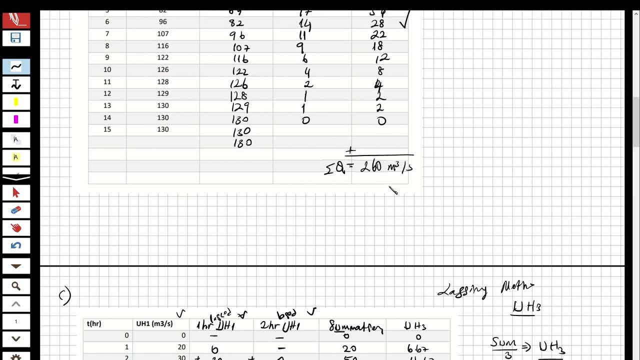 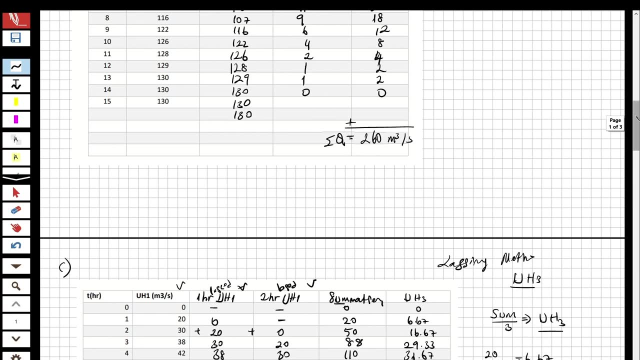 total discharge. if you get the summation of this also, you are going to obtain the same value, but for this one it is. there is no any decimal. so I just take the unit hydrograph for one hour. okay, you can take the summation of this one also. so now let's do it for this one. we.